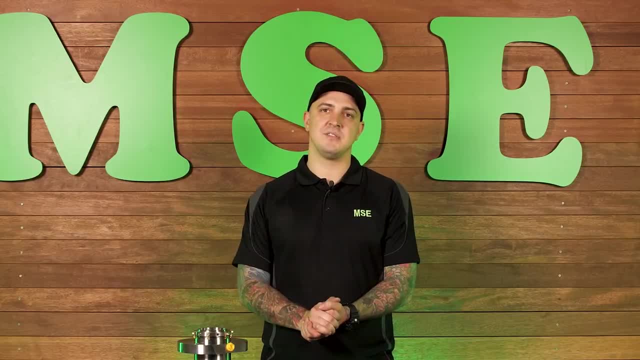 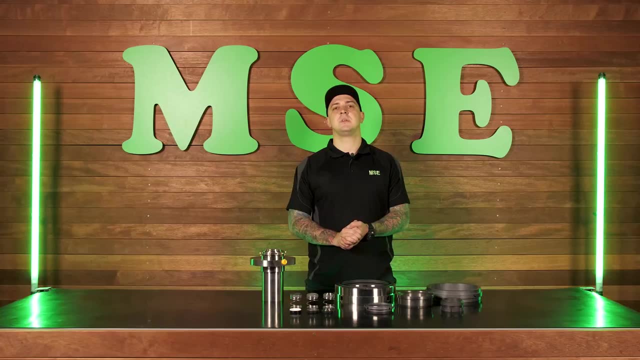 are more material options, but these are the most common ones that I'll be focusing on. Carbon trubbing nitrile is the entry level material combination extremely common in the lower end of the market for water pumps In a clean environment. they work great If 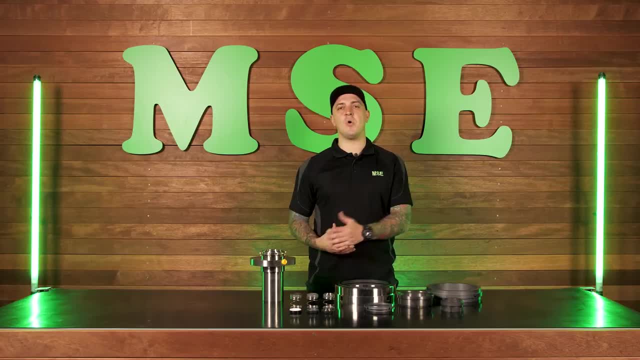 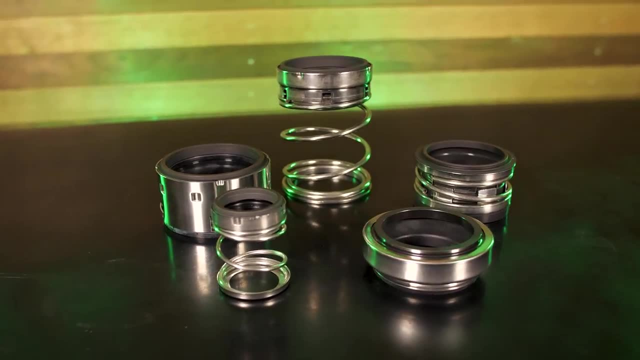 you start getting particles or contaminants, there's a risk of wear because carbon is quite a soft material. Carbon is a black material, often confused with silicon carbide, which has a blue-grey tinge. Ceramic seal faces are prone to cracking under heat, stress or 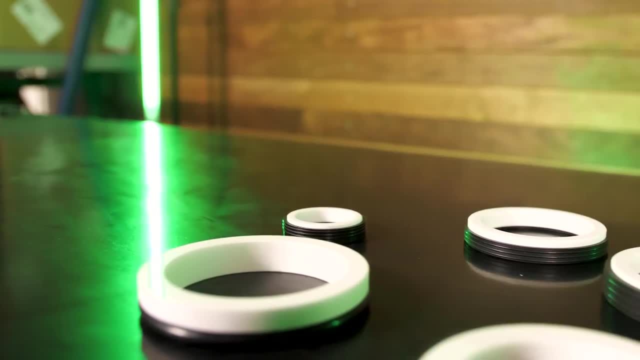 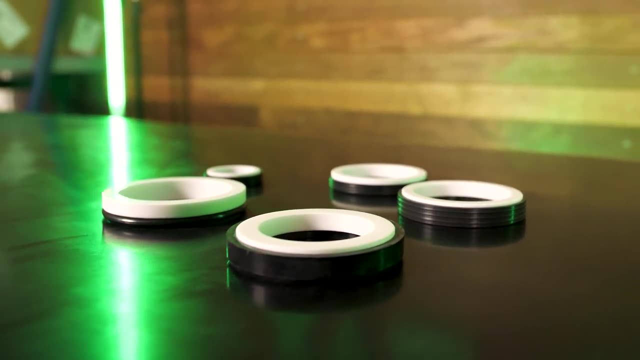 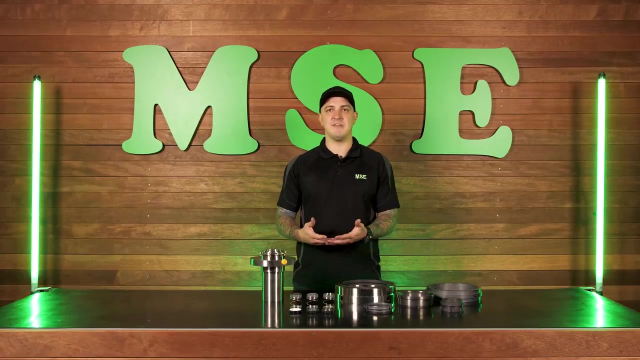 heat fluctuations. These fluctuations can be caused by intermittent dry running or over pressurising the stuffing box, causing excess friction on the seal faces. Ceramic is usually a white or a cream colour. Silicon carbide is a very hard material that can be matched with another silicon carbide face or a carbon face. It is a very hard wearing face and can 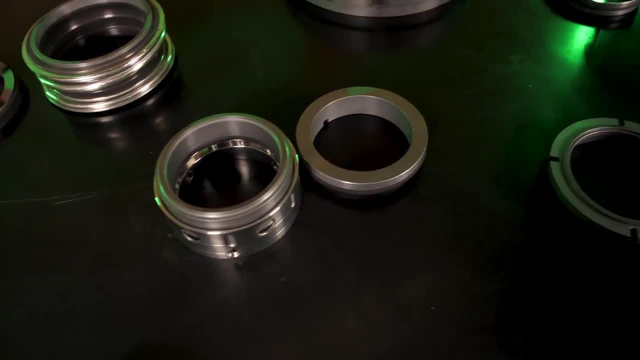 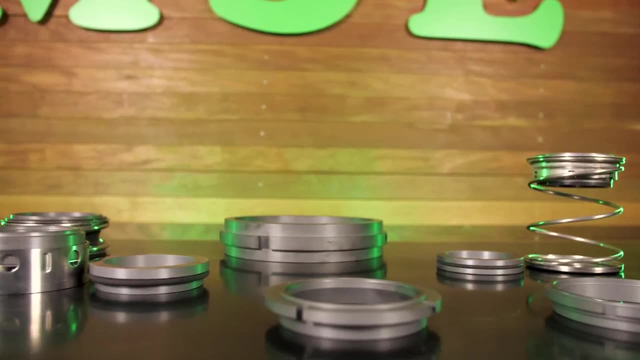 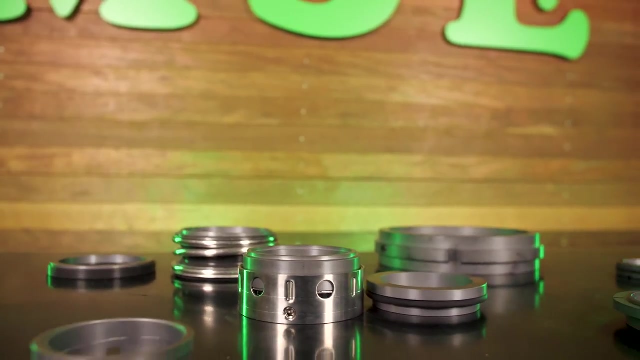 handle a lot more abrasives within the product. Silicon carbide is also less likely to break with heat fluctuations Due to a more labour intensive manufacturing process. the price difference is substantial, hence why more cost effective pumps use carbon ceramic. There are two main types of silicon carbide: reaction bonded silicon carbide and sintered. 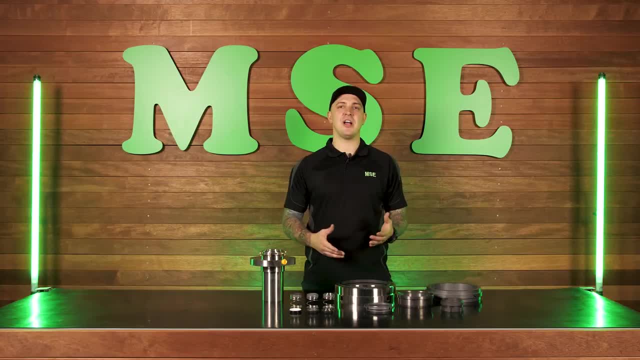 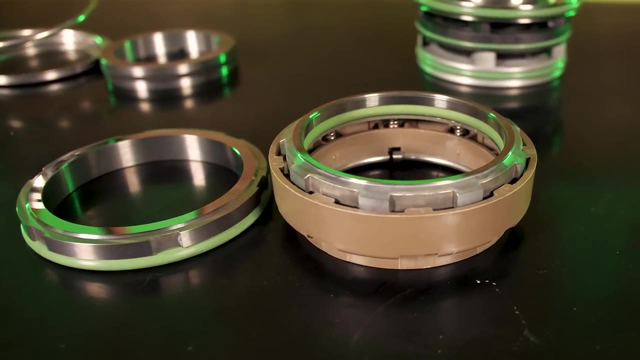 silicon carbide. All of our engineered cartridges use a high grade sintered silicon carbide, as it's a bit harder wearing. Silicon has a blue-grey tinge to it and has a feel similar to glass or ceramic. Silicon carbide is another very hard material and, unlike silicon carbide, it is not brittle. 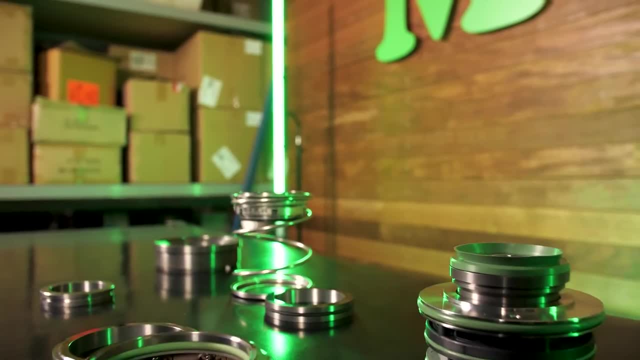 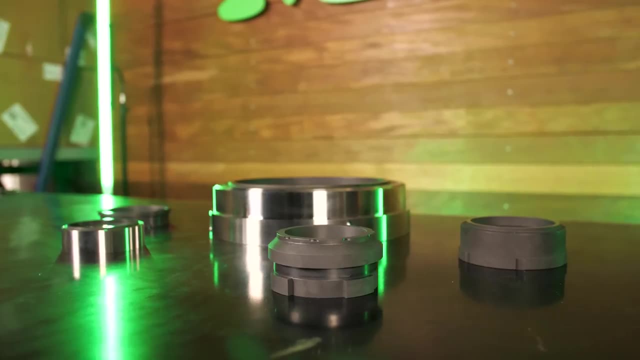 and will not chip or crack as easy. It is an expensive product that is extremely difficult to manufacture. due to its hardness, It has a dark silver metallic look and is very heavy. There are multiple variations of carbon as well, to suit different temperature pressure. 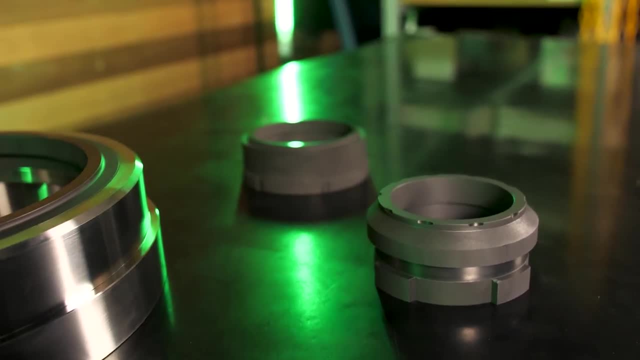 and dry running applications. The most common form of carbon is resin- impregnated carbon. Elastomer choice is also critical, The main elastomers being Viton, Niacinamide and Aluminum. The most common form of carbon is resin impregnated carbon. Elastomer choice is also critical. 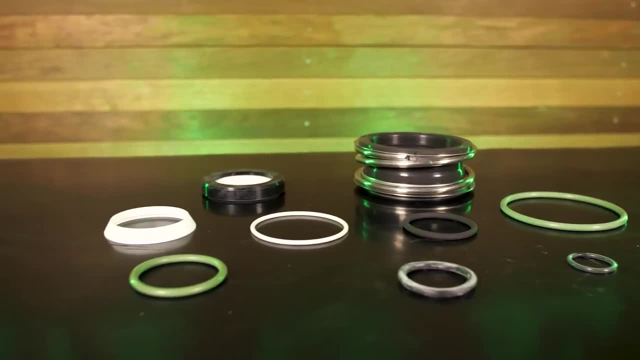 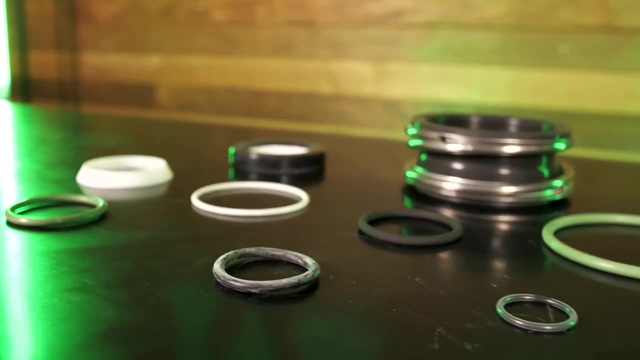 The main elastomers being Viton, Niacinamide and Aluminum. These can be very specific to the application, depending on temperature, pressure and chemical makeup of the product, The main elastomers being Viton, Niacinamide and Aluminum. Different elastomers can be toxic and not suitable for the food industry. 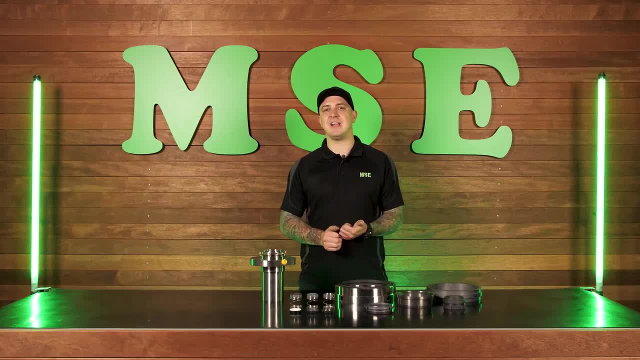 Part of this main elastomer choice is the彩. In more demanding applications, we can also supply AFLAS, COWRES and FEPO rings. Next, iscard, which can be quite simple and cost effective. Last is a very basic one, which is a separate version of a range daggers.